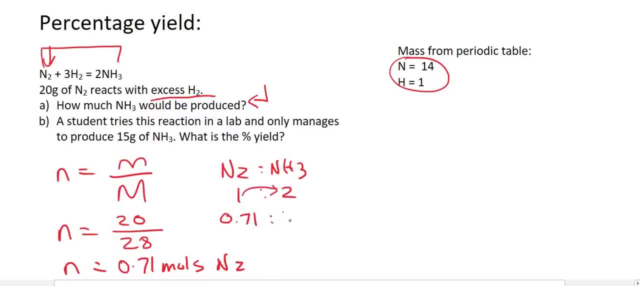 0.71, then I multiply by 2 and that's going to give me 1.42.. So therefore we have 1.42 moles of NH3.. Then we can work out the NH3 mass. Sorry, it says here how much NH3. I should have said what. 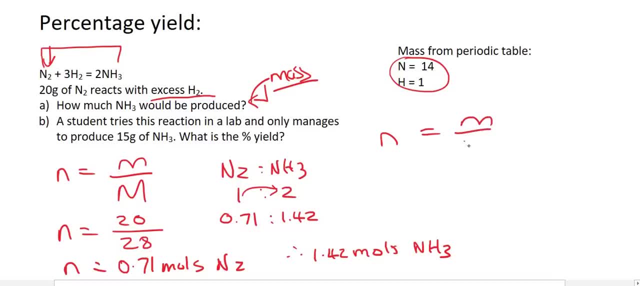 mass. What mass is going to be produced? So we use this formula and now we have the number of moles. The molar mass of NH3 is 1 nitrogen and 3 hydrogens, And so if you go do all the calculations there, you're going to end up with a mass of 24.14 grams. Okay, so we formed 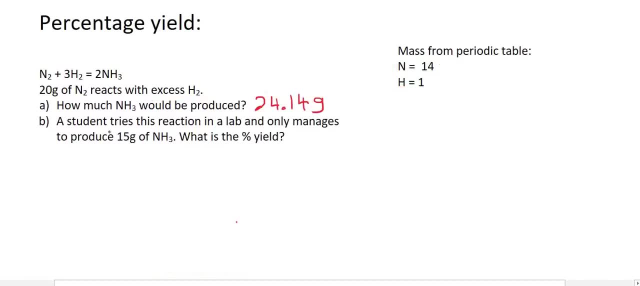 24.14 grams. Then it says: a student who obviously just really loves chemistry and just gets home and doesn't want to do anything else but just go practice some chemistry, tries this reaction in a lab, but they only managed to produce 15 grams. What is the percentage yield, Guys? so this 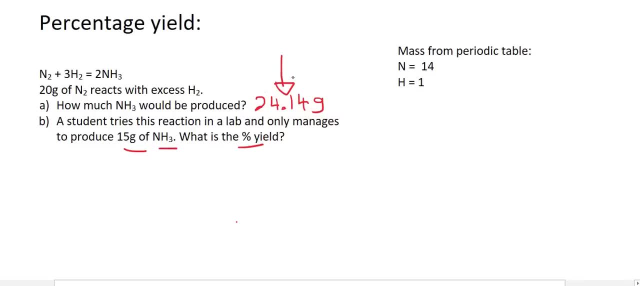 24.14,. that is a theoretical amount. It's the amount that we should be able to form, But in real life, chemists usually form a little bit less. The reason is, is humans- I mean, we're not perfect- We do make mistakes. Maybe we drop a little bit of the powder, Maybe our 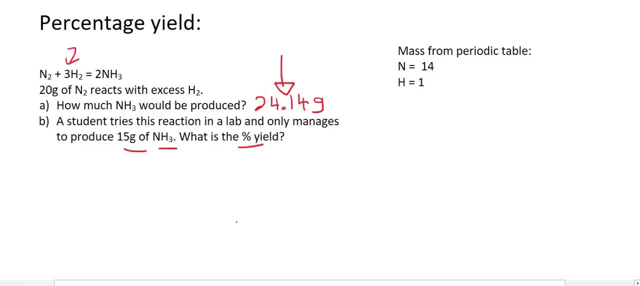 ale is not working so nicely on that particular day. Maybe our nitrogen and hydrogen are not very pure. The point is, is that as humans or in real life, you won't be able to form as much as 24.14.. I mean, maybe you can if you get it perfect, but most times you're. 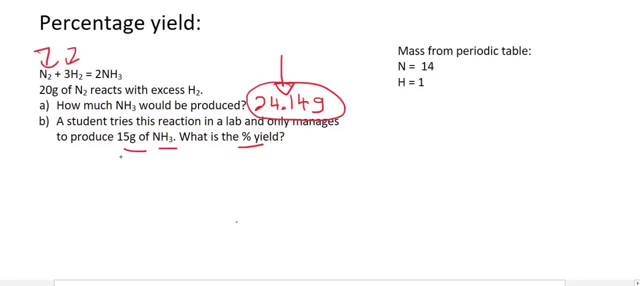 going to get a little bit less. So when this student tries that, he only, he or she only manages to form 15 grams. So what is that as a percentage? Well, the percentage yield is always equal to your actual, or your actual yield divided by theoretical. Now, theoretical: 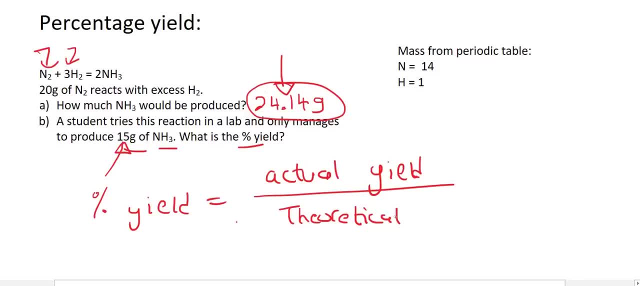 is how much you could form in theory, So like if everything works perfectly, how much would you form, And so the actual yield is 15.. The theoretical is how much you would form if everything was perfect, And that's 24.14.. And so you can work out this person's yield. 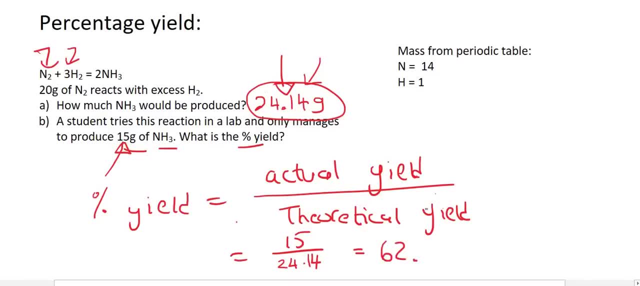 And it's about 62%- 62.1.. If we round up it's going to be about 1- 4%, because we should times by 100.. I forgot about that. So you can say that this student had a success rate of about. 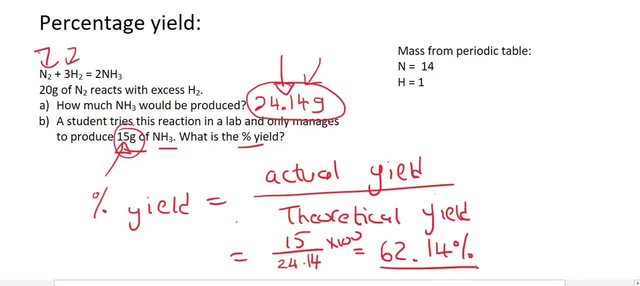 62%. If the student did everything perfect, then the success rate would be 100%, But because there was a little bit of error, the success rate was about 62%. Okay, so that is what percentage yield is. you can think of it as your success rate. 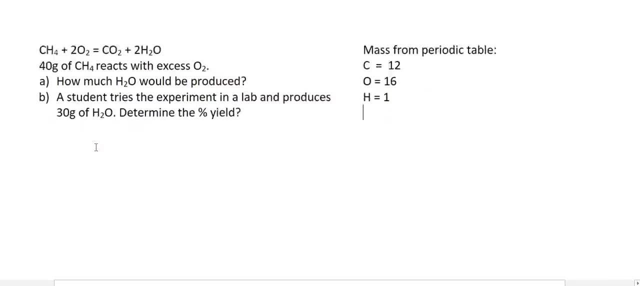 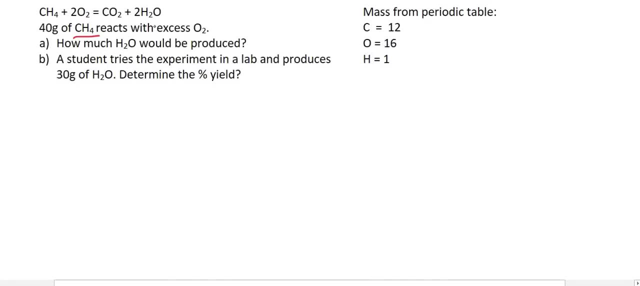 Here's another one, So maybe you want to pause this video and give it a go. It's very easy. So we are told that 40 grams of CH4 reacts with excess oxygen. the excess is just telling us we don't have to worry about limiting. The only time we have to worry about limiting. 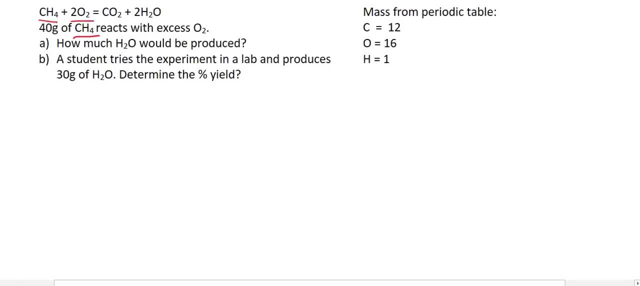 is when they give you information about the CH4 and the oxygen. then you need to worry about limiting. Okay, so how much water would be produced? So this is a very easy question. But now you guys are like geniuses at this, I'm sure, So we can work out the number of. 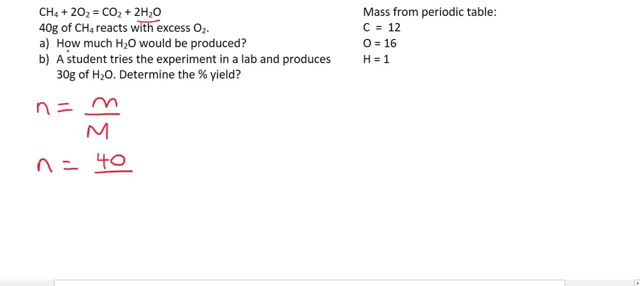 moles, The moles of CH4, because they've given us the grams, the molar mass of CH4, well, it's one carbon, so that's 12, plus four hydrogens, so that's going to be plus four. And if you 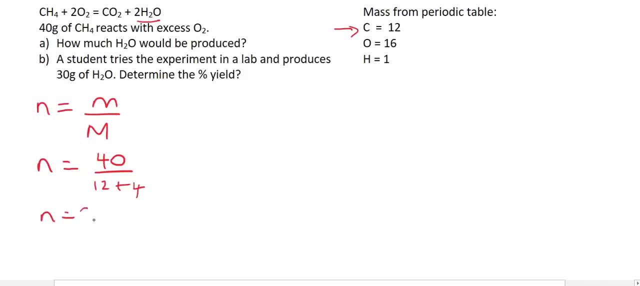 go work that out. you're going to get 2.5.. It's a nice number, 2.5 moles of CO2.. Where am I getting CO2 from? Oh, there is a CO2 there. That's not too bad. CH4.. All right. 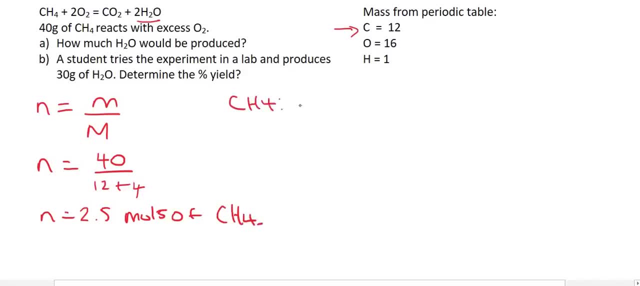 now we can look at the mole ratio between CH4 and H2O. From the equation we can see that it's a one to two. So we can say a one to two ratio. So how much CH4 do we have? 2.5.. So to go from the one to the other, you multiply by: 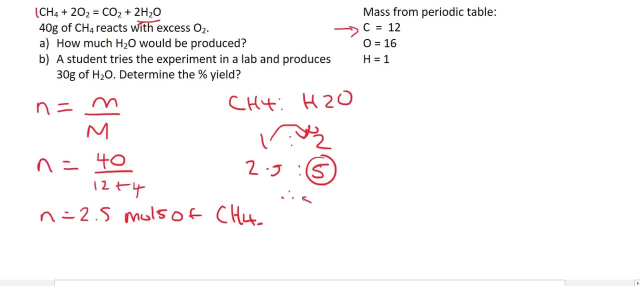 two. So if we multiply by two we're going to end up with five. Therefore we have five moles of H2O. So we could work out the mass using: N equals to M over M again, where the number of moles is five And the molar mass of water is two hydrogens and an oxygen. So 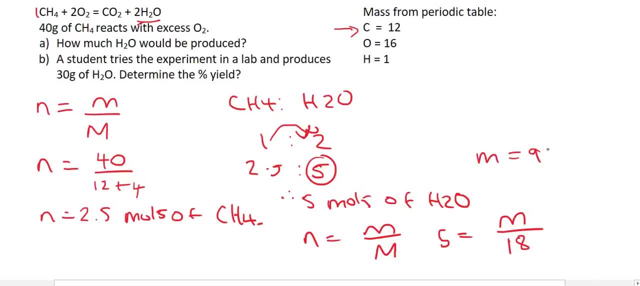 that's 18.. If you go work this out, you're going to end up with 90 grams of H2O. That is the best case scenario. That is how much you would form in real life if you did everything perfectly. However, a student who goes home and tries to do this in a laboratory, they 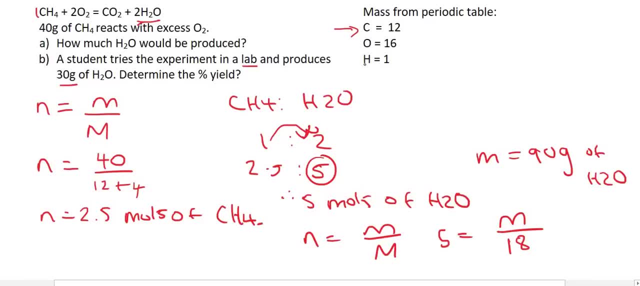 only produce 30 grams. Wow, that's not so good. So what would their percentage yield be? Well, the percentage yield is like your success rate, So it's the actual that you formed. It's divided by the theoretical and then times 100.. Guys, the way to think about this. 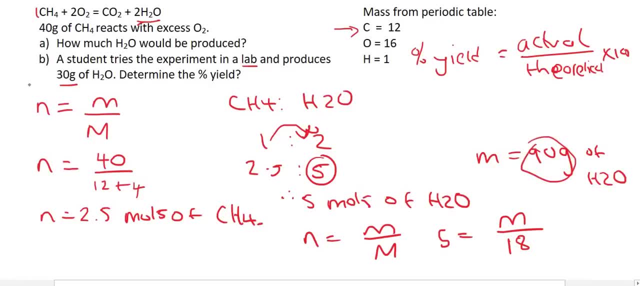 is the highest you could ever get in a test is 90. When you went and wrote your exam, you had a fantastic exam and you got 30 out of 90. That's terrible. So that's going to be 30 out of 90 times by 100, not 900, 90. And that gives you a percentage of 33.33. 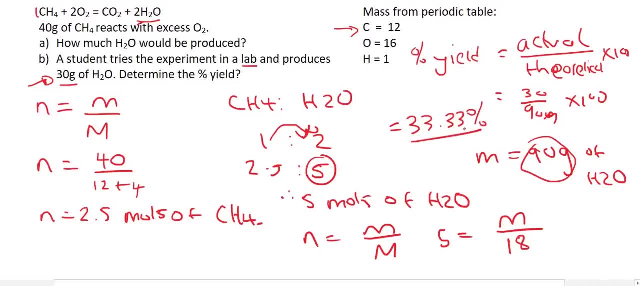 So the student success rate was not very good. It was about 33 percent. So maybe the student was not very good, Maybe the scale that they used to measure everything wasn't very accurate, Maybe the starting material was not very pure, Maybe the student dropped a little bit of. 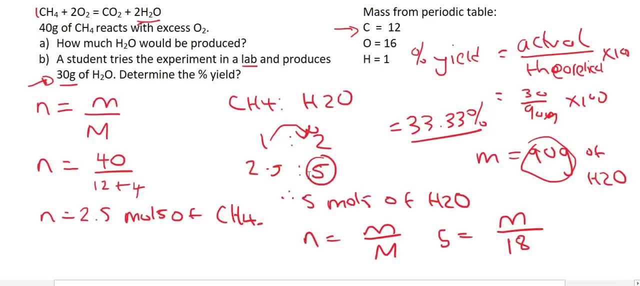 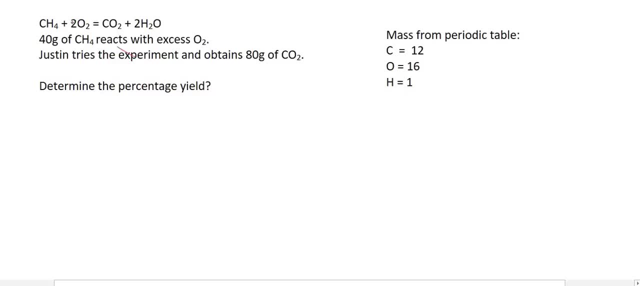 powder on the floor, You never know. There's a whole bunch of reasons that could cause that, But their success rate was 33 percent. Here's another one. Okay, This is the same type of principle, but they're asking this in a little bit of. 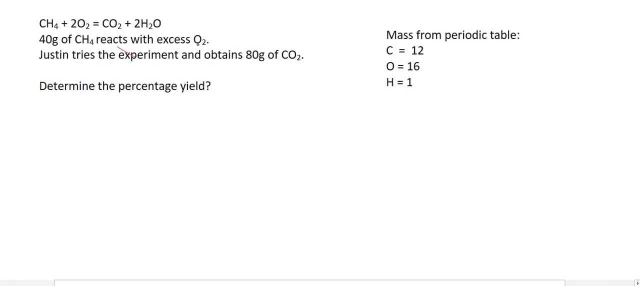 a different way. So they're telling us that 40 grams of CH4 reacts with excess oxygen. When Justin goes home and tries the experiment, he only obtains 80 grams. So would this be the theoretical or the actual? Well, when it's done in real life, that's actual. So 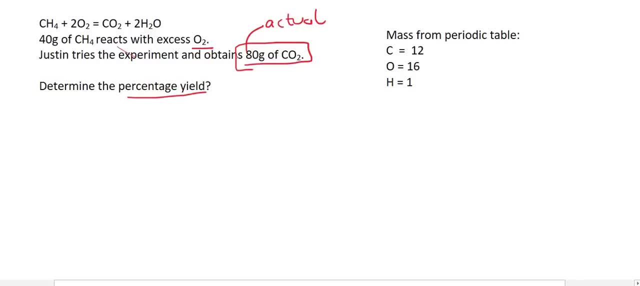 in this question it says you determine the percentage yield. So we know that when Justin goes home he obtains 80 grams of CO2.. Let's see how much CO2 you would be able to form if everything went perfect. So let's go work out the theoretical amount So we can convert. 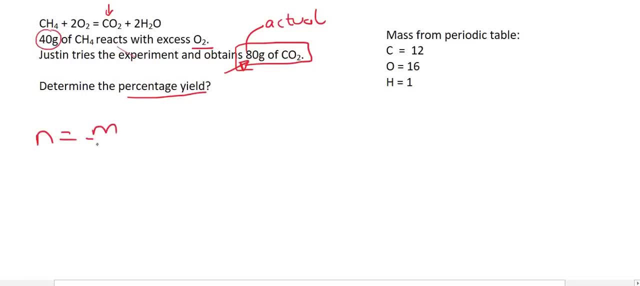 this 40 grams of CO2 into 80 grams of CO2.. So we can convert this 40 grams of CO2 into moles by using: n equals to m over m, And so the number of moles would be 40 over the. 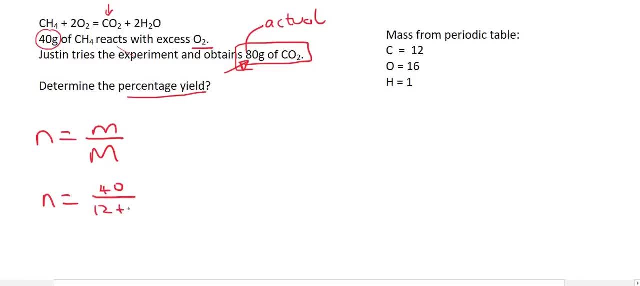 molar mass of CH4, which is going to be 12 plus 4 hydrogens. That's 12 plus 4.. And so that's going to be 40 over 16.. Let me just get the answer without writing all these steps. 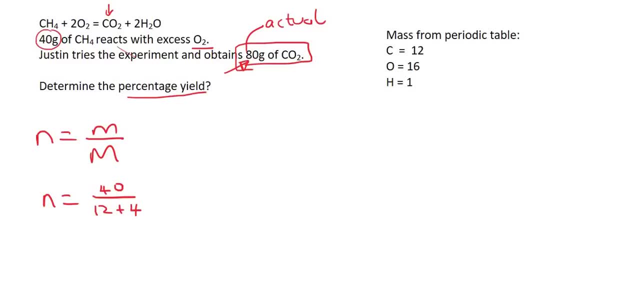 So 40 over 16 is going to give you 2.5.. Oh yes, Another nice number: 2.5 moles, And that's CH4.. Now let's see how much. Okay, So Justin got 80 grams of CO2.. So let's work out the. 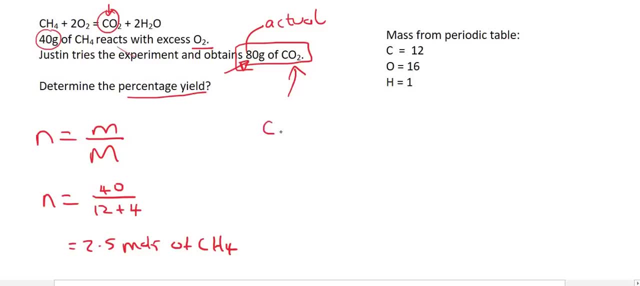 CO2.. So the mole ratio of CH4 to CO2 is 1 to 1.. So 1 to 1. The number of CH4 is 2.5. And so the CO2 would also be 2.5, because it's a 1 to 1 ratio. Now we can work out the mass of CO2 by using this. 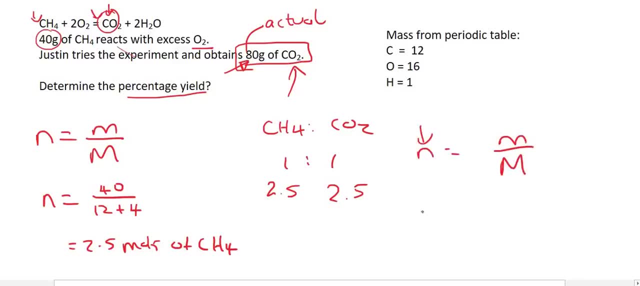 formula, And so the number of moles is 2.5.. The mass is m, The molar mass of CO2,. well, it's one and then two oxygens. So it's 16 plus 16, which is 32.. If you go work that out, you get 110 grams. 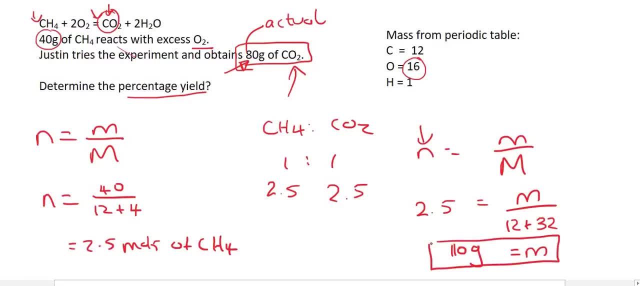 That makes sense In theory. you should always form more, So in theory you should be able to form 110 grams. When Justin goes home, he forms 80 grams. That's not too bad. He's not too far off. 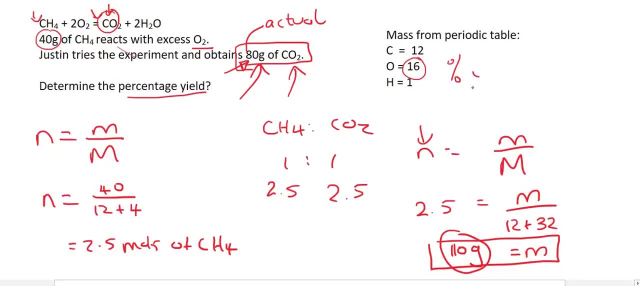 So let's see what his success rate is. So the percentage yield is your actual, which is what amount which is in the ideal scenario, And I don't actually think he did too bad. He got 80 out of 110 times by 100. And so his success rate is 72.73%. Not bad, Okay. so he got about 72.73%. 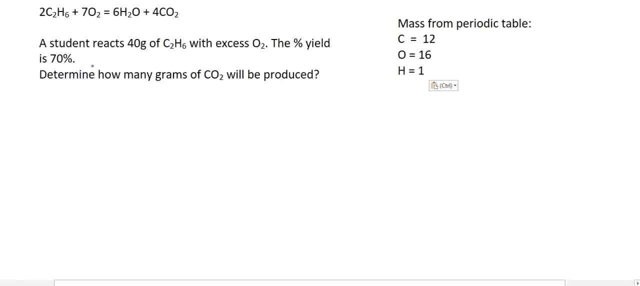 success. Last question for this lesson, guys. So here they say that a student reacts 40 grams of C2H6 with excess. The yield is 70%. Aha, So what that means is that the success rate is 70% And 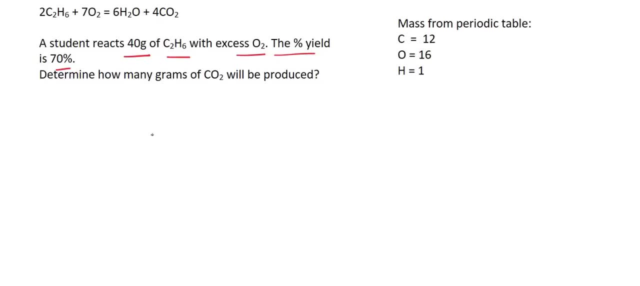 the success rate is 70%. Okay, Determine how many grams of CO2 will be produced. Okay, So let's first work out how much CO2 would be produced if everything went perfectly. So this is under the ideal situation. So let's go convert the 40 grams of C2H6 into moles, So that's 40. Well, 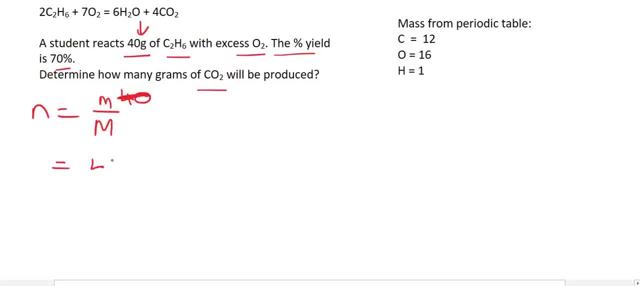 let's first write out the formula, Kevin, And that's going to equal 40 over. Now the molar ratio, I mean the molar mass of C2H6, is C2.. So that's two carbons, That's 24 plus six, because 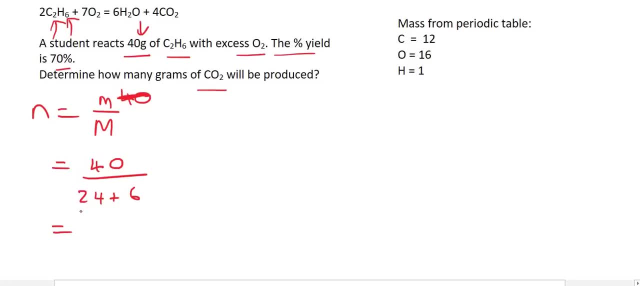 six hydrogens, And so that's going to give us 40 over 30,, which is 1.33 moles, 1.33 moles of C2H6.. So how much carbon dioxide should we be able to form? Well, let's look at their ratio. So the 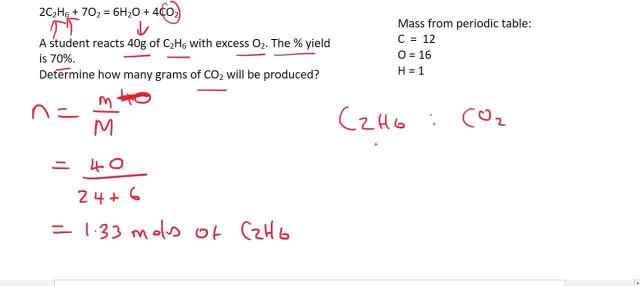 ratio between C2H6 and CO2 is C2H6.. And so that's going to equal 40 over 30,, which is 1.33 moles of CO2.. And so that's going to equal 40 over 30,, which is 1.33 moles of C2H6. And so that's going to 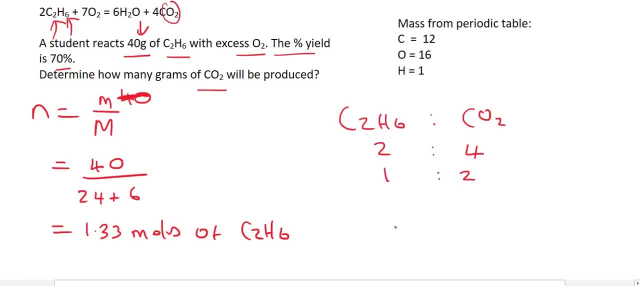 I'm going to quickly simplify that to a one to two. Now, how much C2H6 moles do we have? 1.33.. So if we times that by two, then the CO2 should be 2.66.. So let's see how much mass that would be. 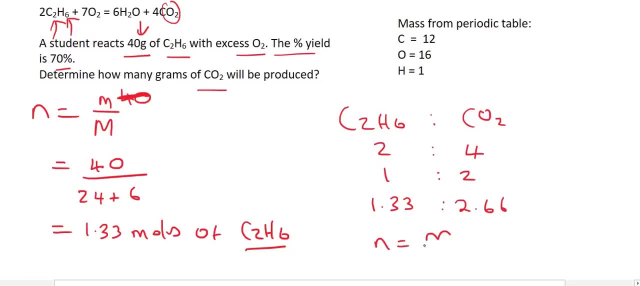 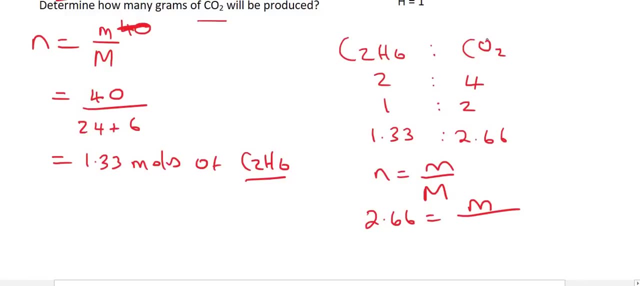 2.66 moles of CO2.. We could use this formula: And so 2.66 equals to the mass over the molar mass of CO2, which is 12 plus 30.. 1.33 moles of CO2.. And so we get 1.66 moles of CO2.. And so we get. 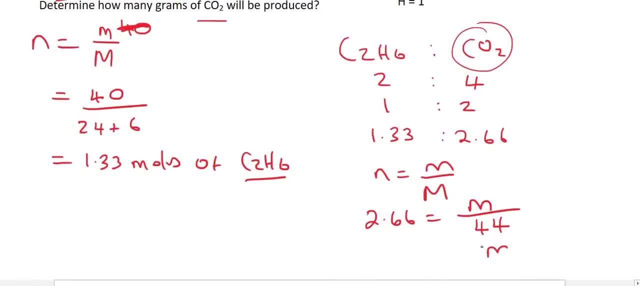 plus 2 oxygen, And so that's going to be a total of 44. And if you go work out the mass, that would be 117.04 grams. That is the best scenario that you could ever have. That is theory. When one of 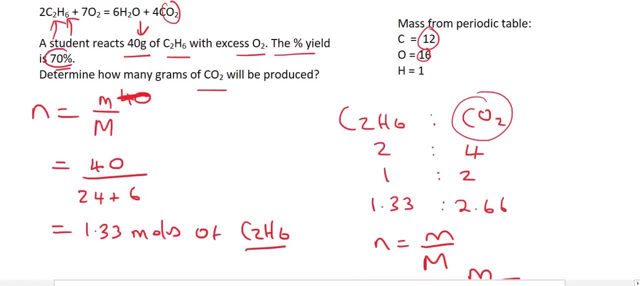 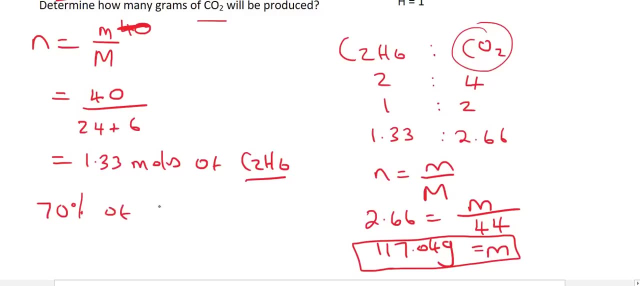 our students went and did the reaction. they got a success rate of 70%. So to work out the mass that they acquired, we could work out what 70% of 117.04 is, And so that's 70 over 100 times by 117.04.. 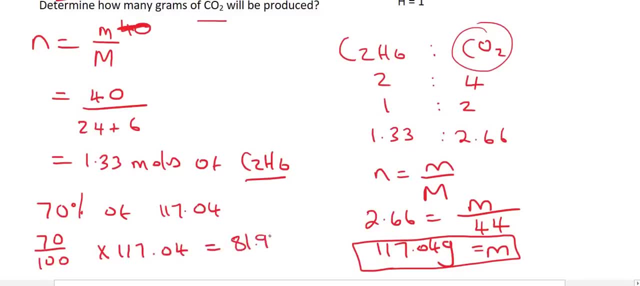 And that's going to give us a success rate of 81.93 grams. So the best, the most amount of mass you would ever be able to form from this experiment, is 117.. This student who attempted it had a 70% success rate, So they formed about 81.93. 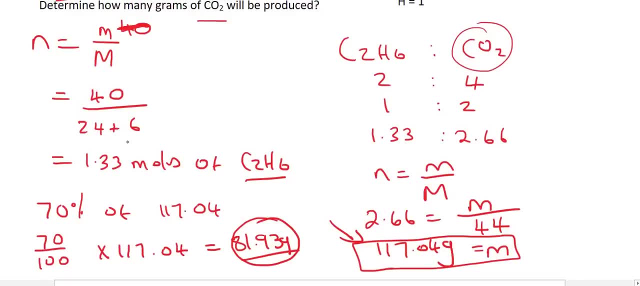 Guys, that's the end of this lesson. That is how you work with percentage yield. Thank you very much.